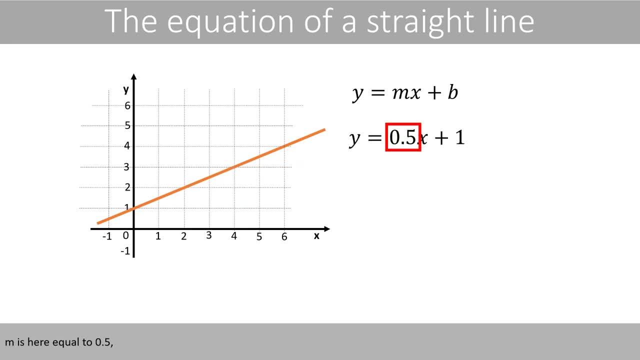 m is here equal to 0.5, and b is equal to 1.. For example, the following horizontal line intercepts the y-axis at 3, and has a slope of 0. Since m is equal to 0,, the equation is y equal to 3.. 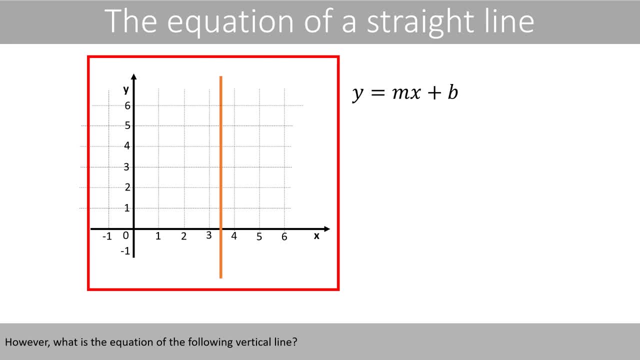 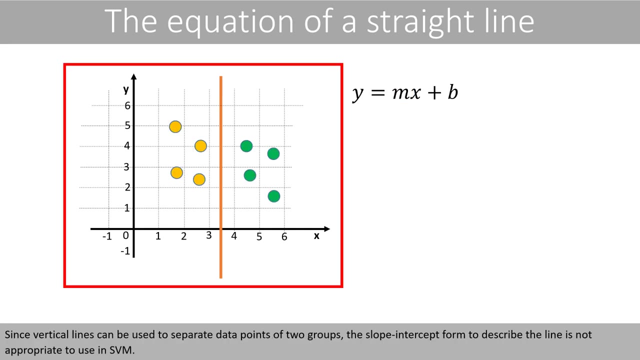 However, what is the equation of the following vertical line? It turns out that this form of equation cannot be used to describe a vertical line, because the slope would then be infinitely large, Since vertical lines can be used to separate data points of two groups. 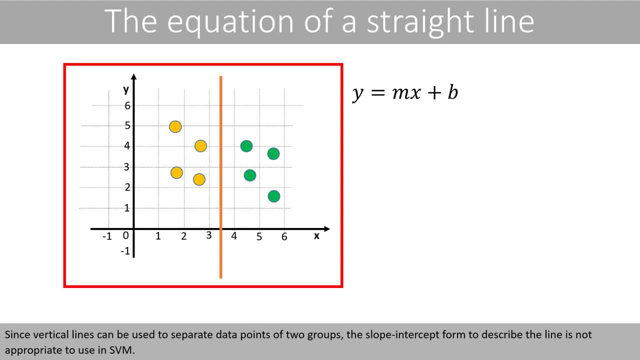 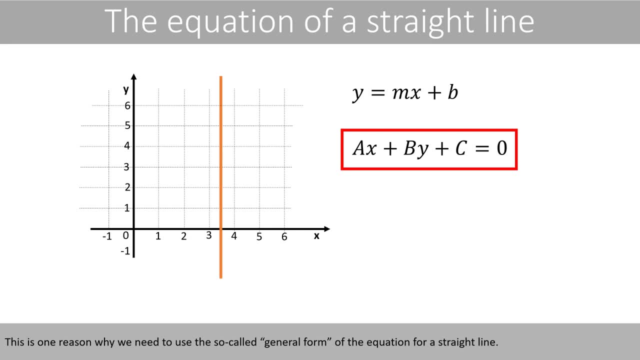 the slope-intercept form to describe the line is not appropriate to use in support vector machines. This is one reason why you need to use the so-called general form of the equation for a straight line If we move these two terms to the right-hand side. 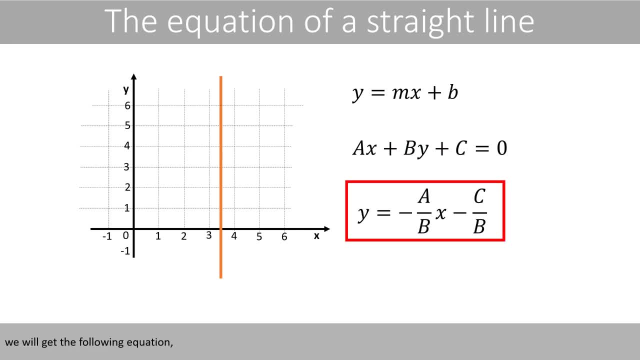 and divide by b, we will get the following equation: where this is the slope of the line and this is the intercept, We can see that the coefficient a affects the slope and the constant c affects the intercept, whereas the coefficient b affects both the intercept and the slope. 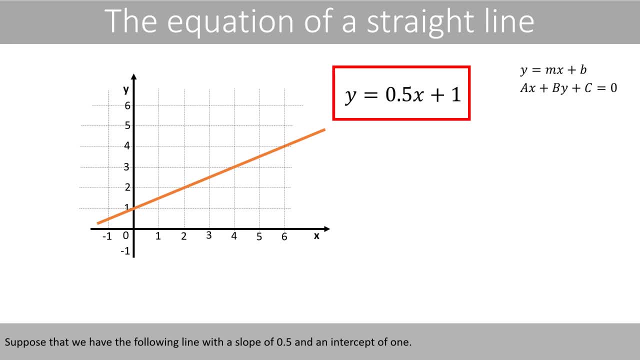 Suppose that we have the following line, with a slope of 0.5 and an intercept of 1.. We will now convert this equation to the general form. We therefore move all terms to the left-hand side like this, To be consistent with this form. 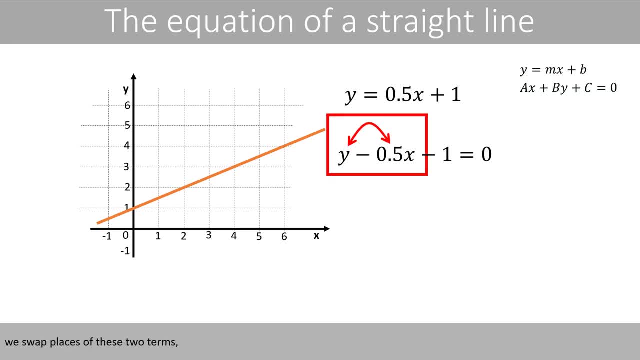 we swap places of these two terms so that we have the following equation that also describes the line. The coefficients are usually expressed as integers. in this form, If we, for example, multiply all terms by 4,, we will get the following equation that also describes the same line: 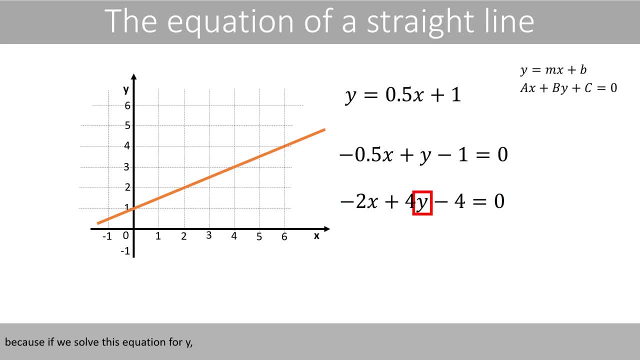 Because if we solve this equation for y, we will end up with the following equation In the general form: one should set the coefficient a to be a positive number, which can be done by multiplying all terms with negative 1, so that we get the following equation that also describes the same line. 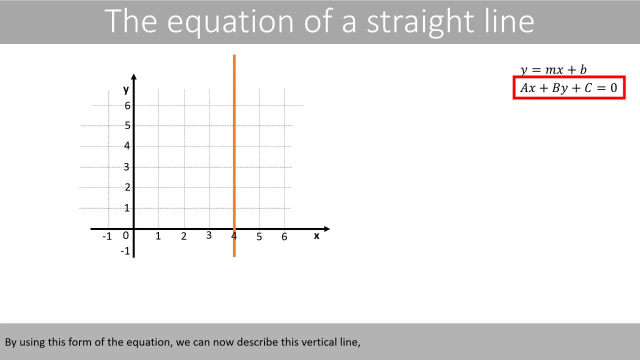 By using this form of the equation, we can now describe this vertical line like this, because x is equal to 4 along this line. Remember that we can describe this line with these two different forms of equations, where we, from here on, will focus on the second type of equation. 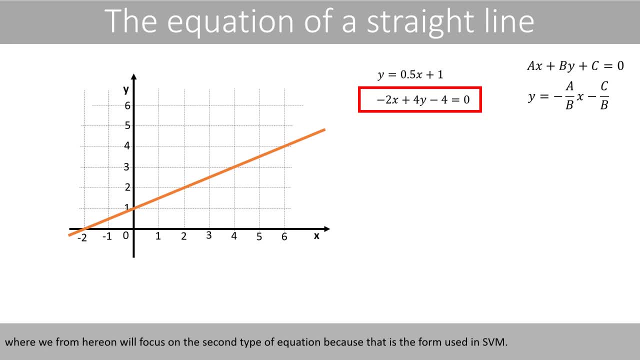 because that is the form used in support vector machines. The coefficient a is equal to negative 2, and coefficient b is equal to 4,, whereas c is equal to negative 4.. Let's plug in these values in this equation. We get the following equation: 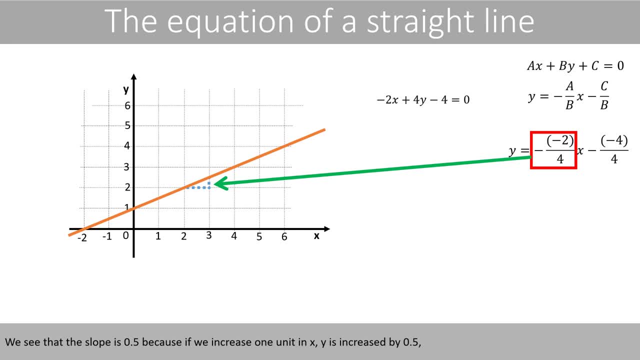 We see that the slope is 0.5, because if we increase one unit in x, y is increased by 0.5. And we see that the intercept is equal to 1.. Linear support vector machines. finds the optimal values of the coefficients a and b. 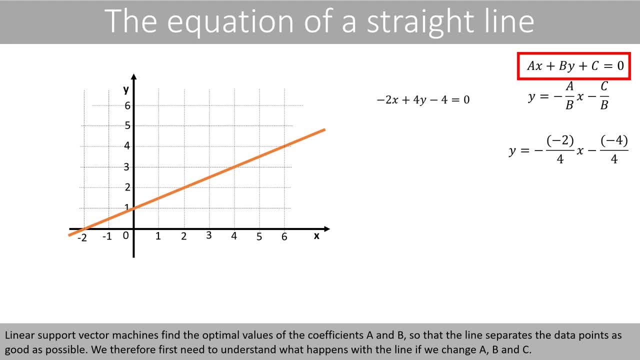 so that the line separates the data points as good as possible. We therefore first need to understand what happens with the line when we change a, b and c. For example, if we increase a from negative 2 to negative 1, the slope will be reduced from 0.5 to 0.25. 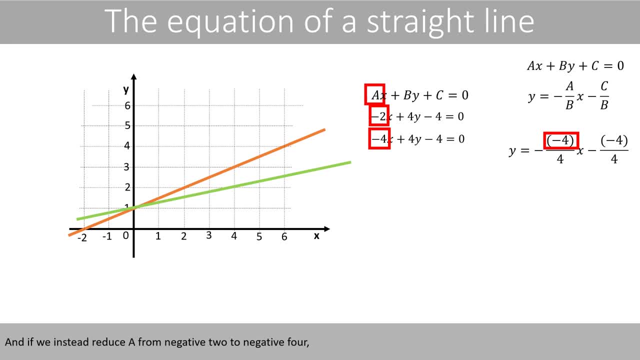 And if we instead reduce a from negative 2 to negative 4,, the slope will be increased to 1.. Note that when we change a, the line is rotating around this point. If we decrease c from negative 4 to negative 8,, 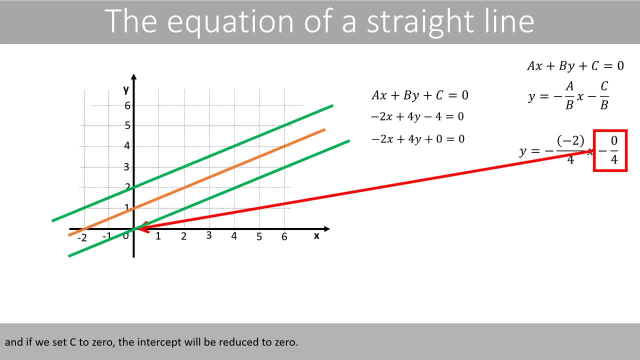 the intercept will be increased to 2.. And if we set c to 0,, the intercept will be reduced to 0.. If we instead increase b from 4 to 8,, we see that the slope is reduced from 0.5 to 0.25,. 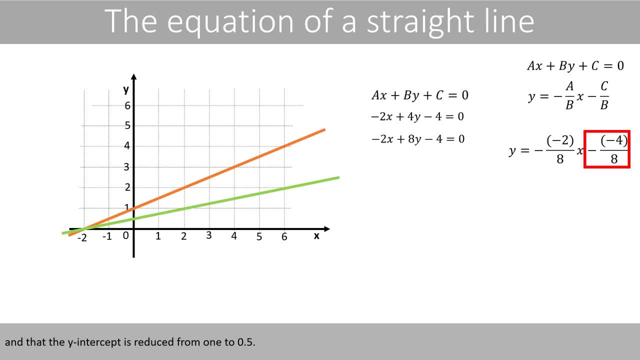 and that the intercept is reduced from 1 to 0.5.. If we now reduce b from 4 to 2, we see that the slope has increased from 0.5 to 1, and that the intercept has increased from 1 to 2.. 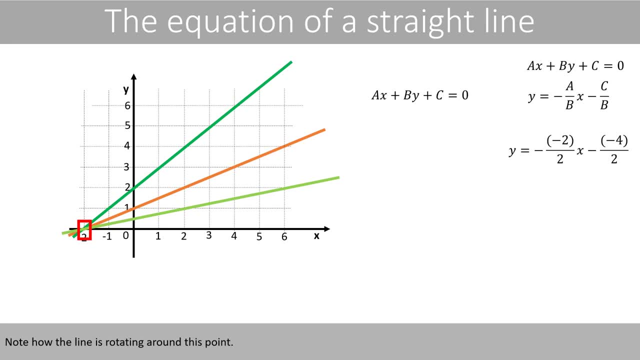 Note how the line is rotating around this point. By changing the values of a and b, we can move around the line like this. Another nice feature about this form of the equation is that it can tell us which side of the line a data point is located on. 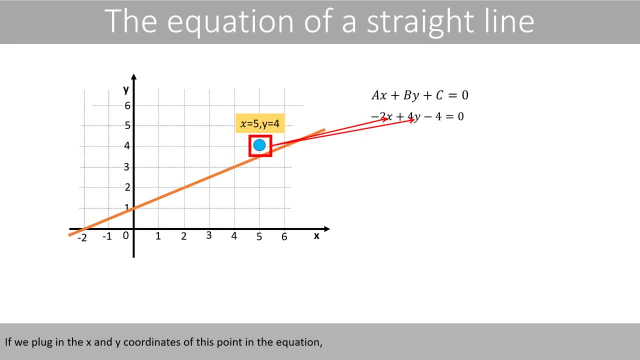 If we plug in the x and y coordinates of this point in the equation, we see that it results in a value that is greater than 0, which in this case means that the data point is above the line. In comparison, this data point results in a negative value. 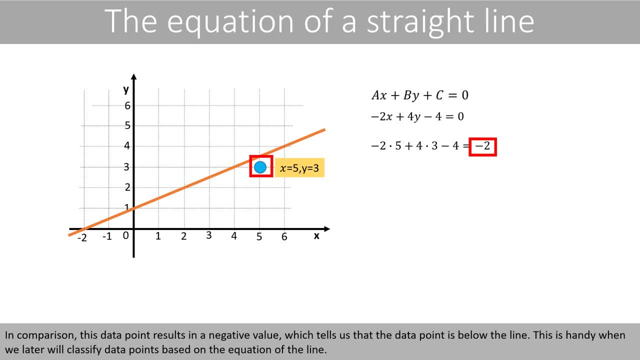 which tells us that the data point is below the line. This is handy when we later will classify data points based on the equation of the line. Note that any data point on the line will result in a value of 0.. Let's see what happens if we add a 1 to the right hand side of this equation. 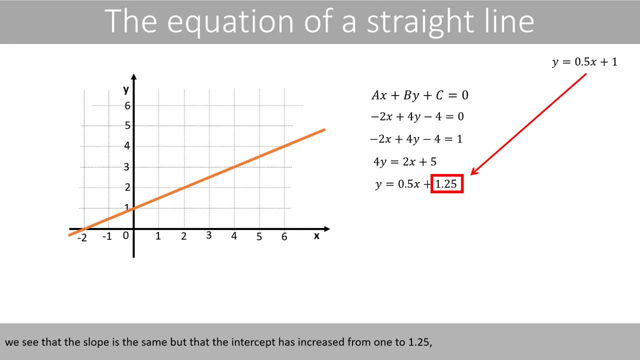 If we then solve for y, we see that the slope is the same, but the intercept has increased from 1 to 1.25, which results in the following line: Similarly, if we add negative 1 here, we will get this line that intercepts the y-axis at 0.75.. 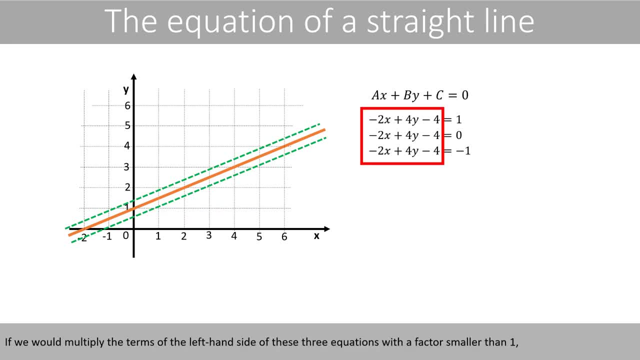 If we would multiply the terms on the left hand side of these three equations with a factor smaller than 1, the green lines would move away from the original line, which stays in the same position, And if we would multiply with a factor greater than 1,. 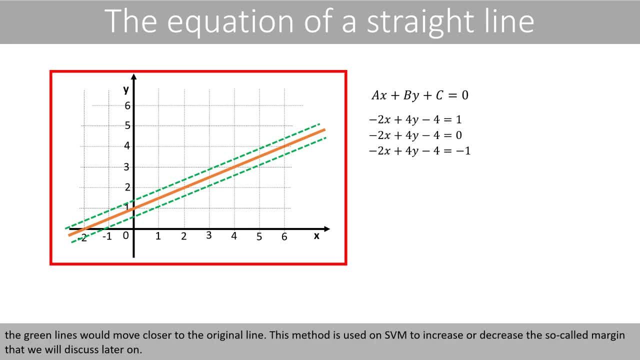 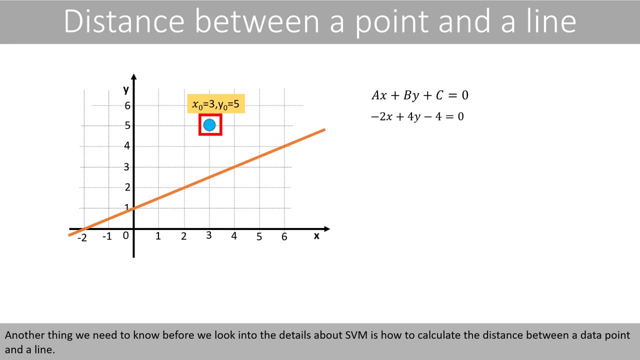 the green lines would move closer to the original line. This method is used in support vector machines to increase or decrease the so-called margin that we will discuss later on. Another thing we need to know before we look into the details about support vector machines is how to calculate the distance between a data point and a line. 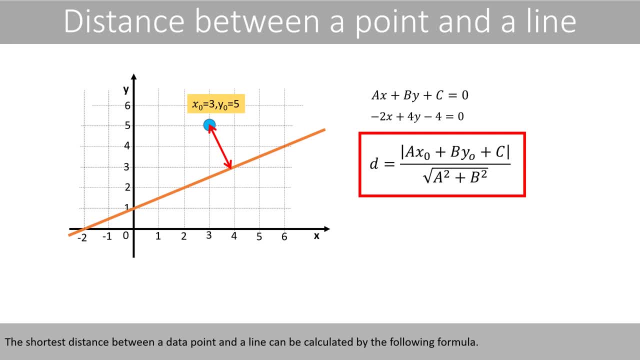 The shortest distance between a data point and a line can be calculated by the following formula: If we plug in the numbers from the equations of the line and the x and y coordinates of the data point and do the math, we see that the distance is equal to y2.24.. 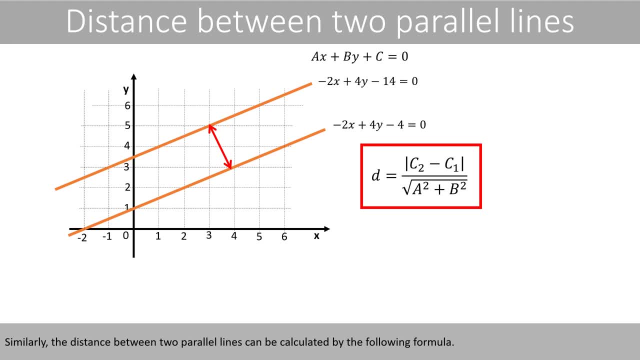 Similarly, the distance between two parallel lines can be calculated by the following formula: If we plug in the coefficients of the equations of the two parallel lines and the constants, we see that the shortest distance between these two lines is about 2.24.. 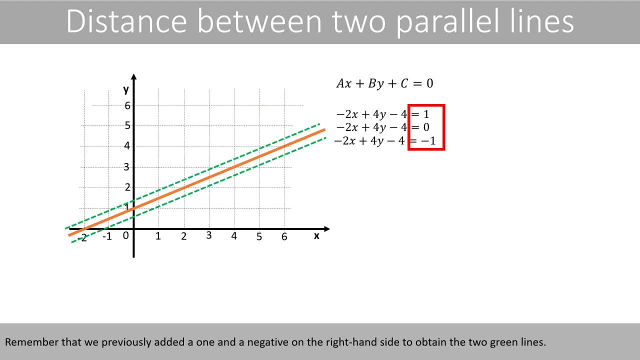 Remember that we previously added a 1 and a negative 1 on the right-hand side to obtain the two green lines. The distance between these two green lines is calculated like this: Note that we have a 2 in the numerator because the absolute difference between the constants. 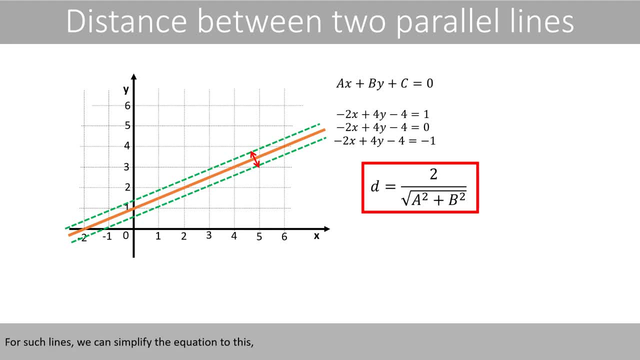 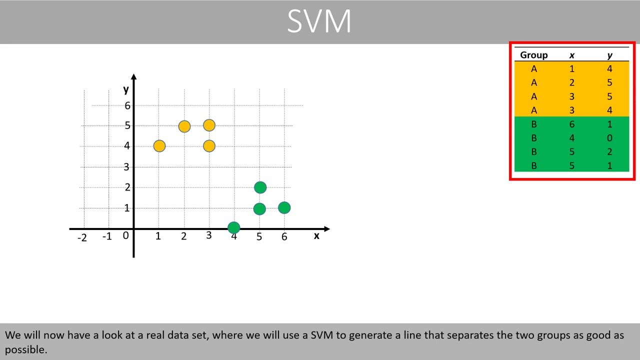 is always 2 for such lines. For such lines, we can simplify the equation to this or like this, which you will see later on. We'll now have a look at the real dataset, where we will use a support vector machine to generate a line that separates the two groups. 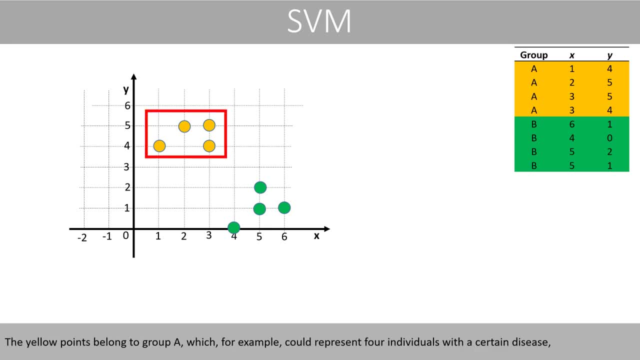 as good as possible. The yellow points belong to group A, which, for example, could represent four individuals with a certain disease, Whereas these green points belong to group B, which could represent healthy individuals, Since we know which group the data points belong to. 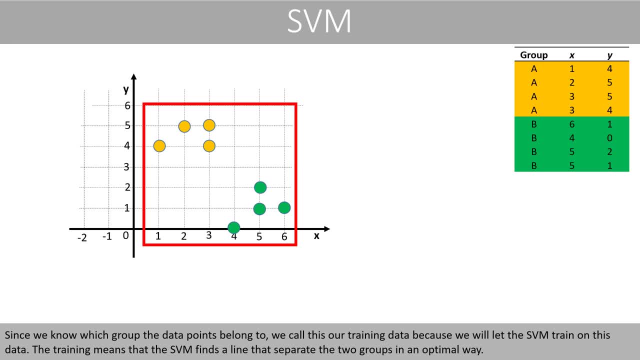 we call this our training data because we let the support vector machine train on this data. The training means that the support vector machine finds a line that separates the two groups in an optimal way. X and Y are two variables that could represent two measurements on eight individuals. 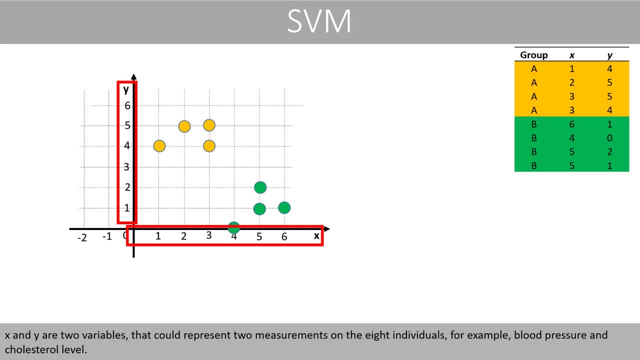 for example, blood pressure and cholesterol level. The following line is the best line to separate the two groups based on the training data. By using this line, we could predict if someone has a disease or not, based on the values of the two variables. If the data point is below the line, 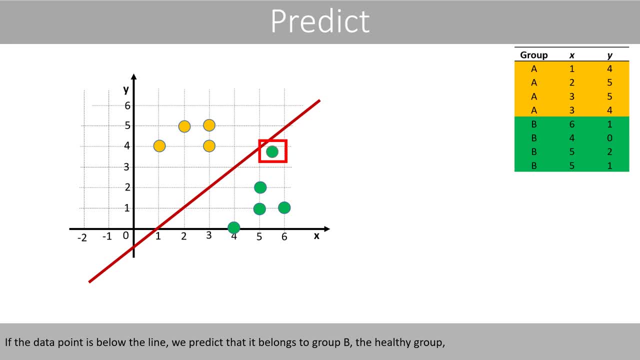 we predict that it belongs to group B, the healthy group, And if the data point is above the line, we predict that it belongs to group A, the disease group, Based on the measured values of X and Y, the blood pressure and cholesterol level. 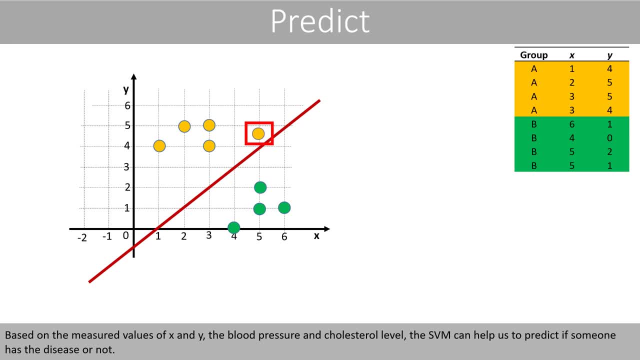 the support vector machine can help us to predict if someone has the disease or not. Note that although this blue line can also separate the two groups completely, it will not be good at predicting new data, because if we would classify the following data point according to this blue line, 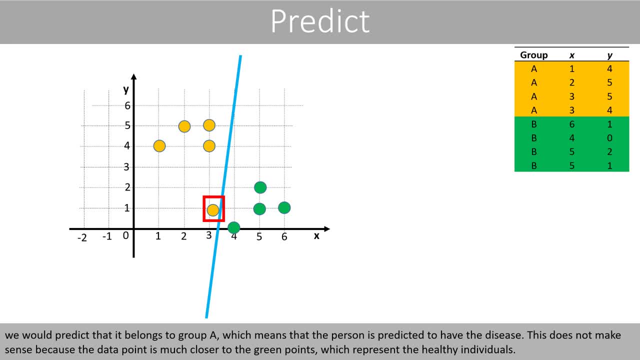 we would predict that it belongs to group A, which means that the person is predicted to have the disease. This does not make sense because the data point is much closer to the green points, which represent the healthy individuals, In comparison by instead using the red line. 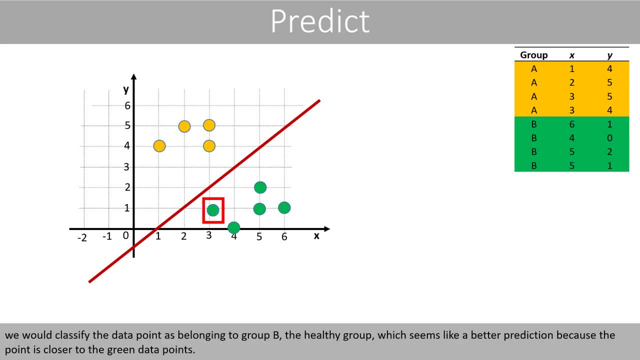 we would classify the data point as belonging to group B, the healthy group, which seems like a better prediction, because the point is closer to the green data points. Note that we here only have two dimensions, but support vector machines work just fine also for several dimensions. 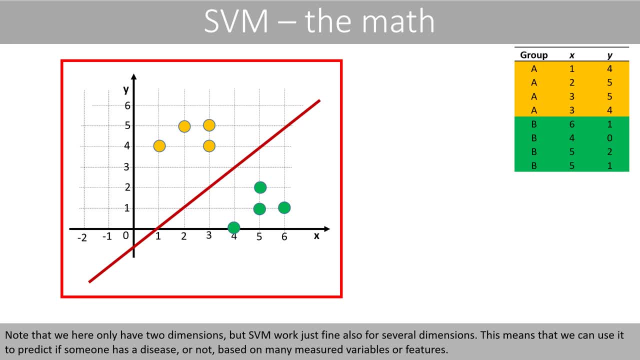 This means that we can use it to predict if someone has the disease or not, based on many measured variables or features. This is the equation of the red line, which has an intercept on negative 1 and a slope of 1.. Let's reformulate the equation. 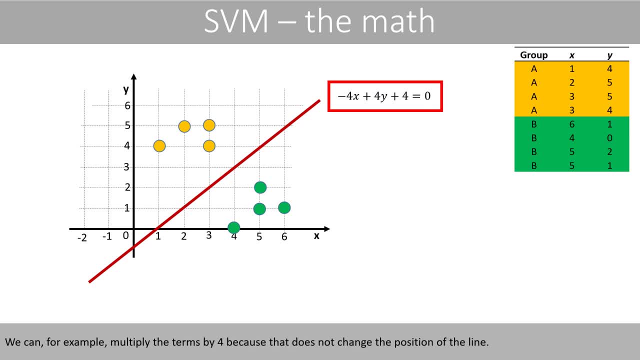 to the form we discussed earlier. We can, for example, multiply the terms by 4, because that does not change the position of the line. Remember that if we solve this equation for y, we'll end up with the following equation: that tells us that the line has a slope of 1. 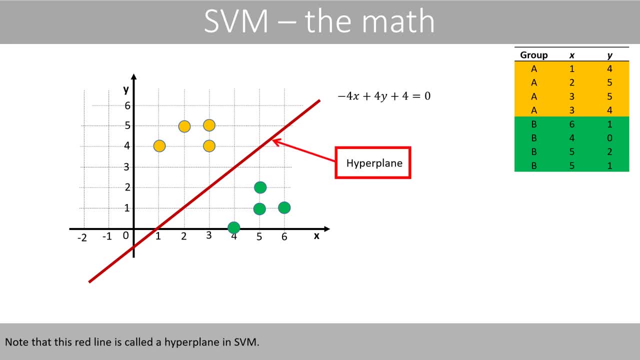 and an intercept of negative 1.. Note that this line is called a hyperplane in support vector machines. We'll now draw two parallel lines that intercept the two closest data points to the hyperplane. Such data points are called support vectors. The equations of these two blue lines look like this: 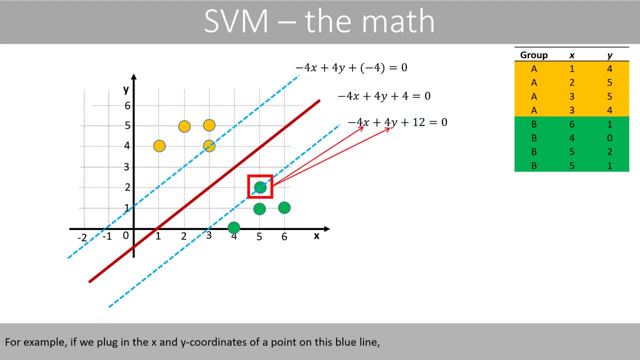 For example, if we plug in the x and y coordinates of a point on this blue line, the left-hand side should be equal to 0, which is true in this case. So can we somehow normalize this equation that represents the hyperplane? 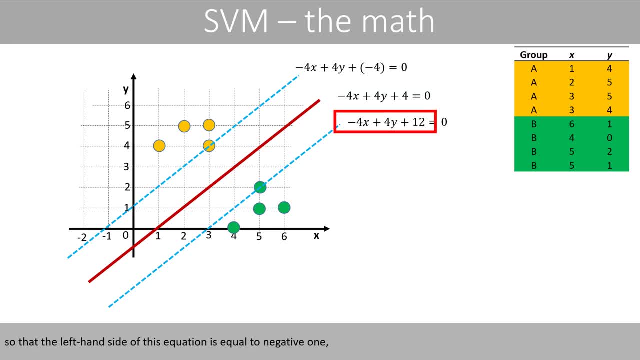 so that the left-hand side of this equation is equal to negative 1 and that the left-hand side of this equation is equal to positive 1,, given that all three equations have the same constant term on the left-hand side as the equation of the hyperplane. 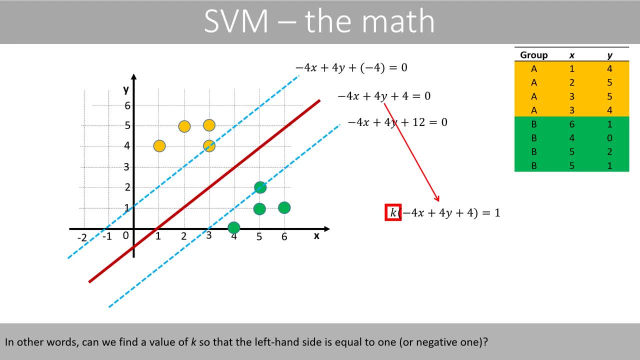 In other words, can we find the value of k so that the left-hand side is equal to 1, or negative 1?? Let's plug in the x and y coordinates of this support vector like this: If we solve this equation: 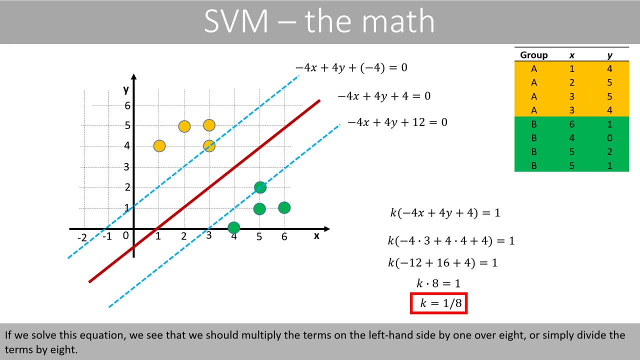 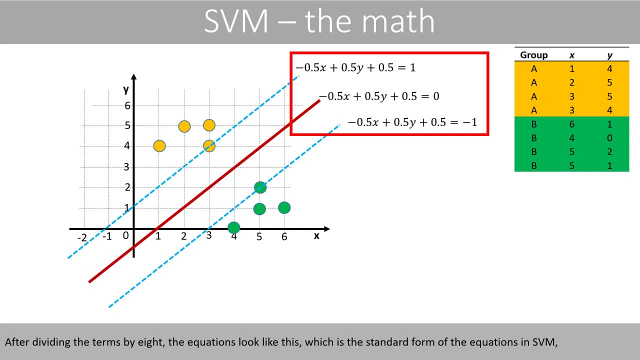 we see that we should multiply the terms on the left-hand side by 1 over 8, or simply divide the terms by 8.. After dividing the terms by 8, the equations look like this, which is the standard form of the equations: 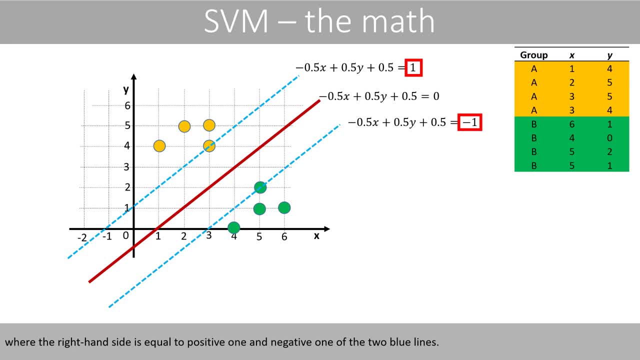 in support vector machines where the right-hand side is equal to positive 1 and negative 1 of the two blue lines. For example, if we plug in the x and y coordinates of an arbitrary point on this blue line, we see that the left-hand side is now equal to negative 1.. 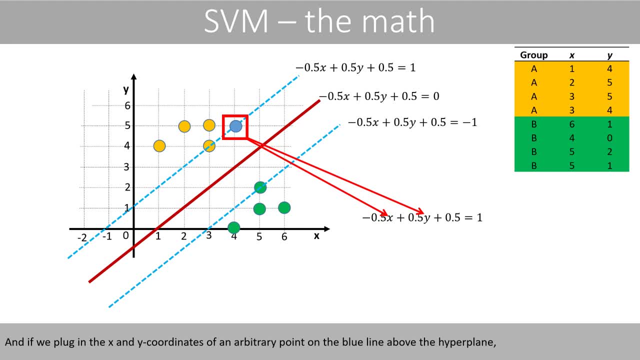 And if we plug in the x and y coordinates of an arbitrary point on the blue line above the hyperplane, we see that the left-hand side is now equal to positive 1.. Let's replace the constant 0.5 with b. Note that the two distances between the red line and our hyperplane 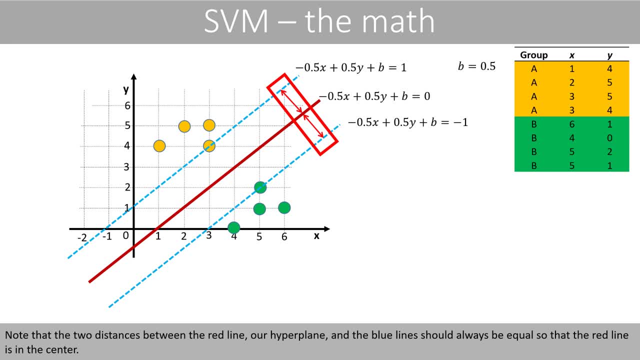 and the blue line should always be equal, so that the red line is in the center. This explains why we use 1 and negative 1 as constants. on the right-hand side, The equation of the hyperplane is usually expressed like this in support vector machines: 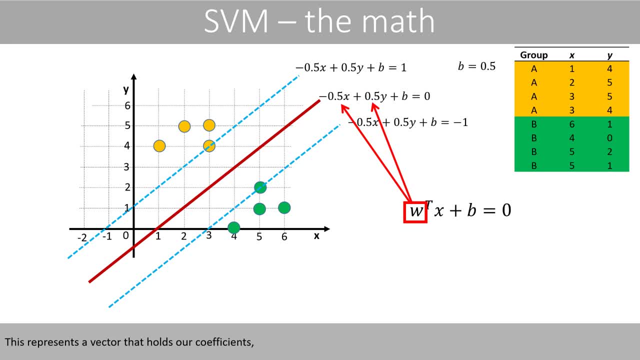 This represents the vector that holds our coefficients, and this is a vector that includes the variables x and y. in our example, t represents that we should transpose the vector w- If we plug in the coefficients- and x and y in this equation, we see that if we multiply these two vectors, 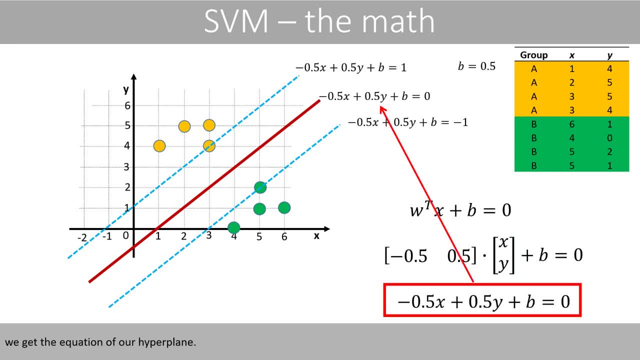 we get the equation of our hyperplane. Note that x in this equation is a vector of the variables x and y. Usually one defines the two dimensions as x1 and x2 in support vector machines instead of x and y. but to keep things simple I have here named the axes x and y. 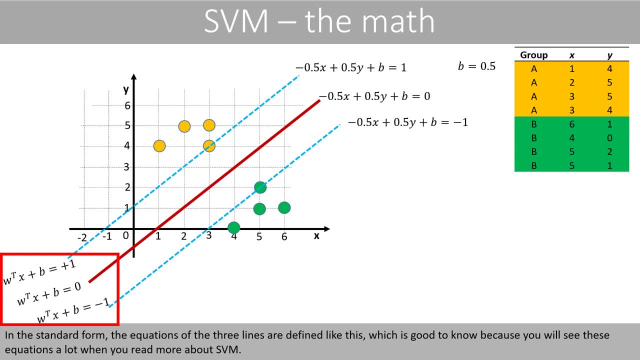 In the standard form, the equations of the three lines are defined like this, which is good to know because you will see these equations a lot when you read more about support vector machines. Now let's use our hyperplane to classify if a data point belongs to group A, the yellow points. 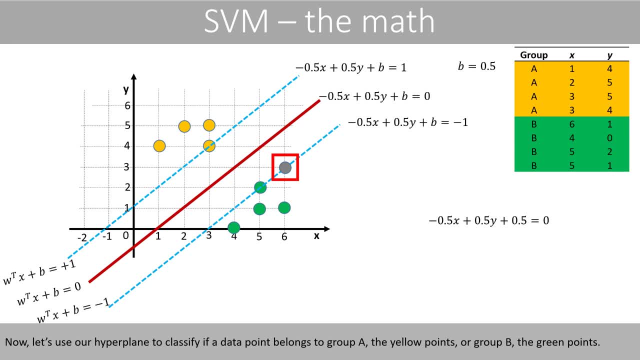 or group B, the green points- We plug in the x and y coordinates of this data point of an unknown class in the equation of the hyperplane. Since this results in a negative value, we predict that the data point belongs to the negative group. 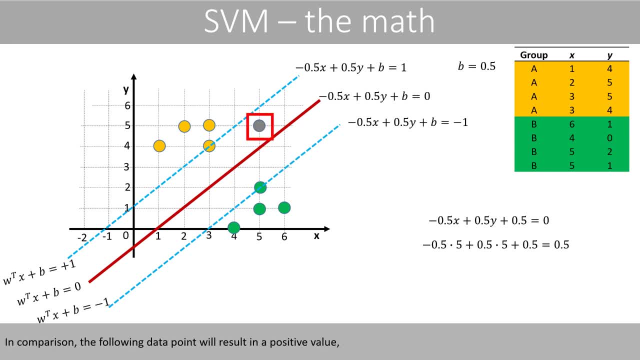 which is group B in this case. In comparison, the following data point will result in a positive value, which means that we predict it to belong to the positive group, which is group A in this case In support vector machines. one therefore divides the two groups. 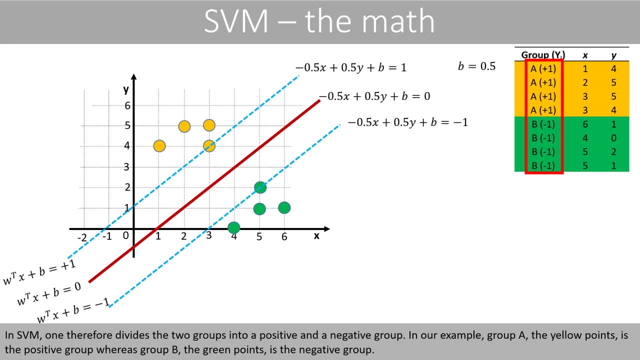 into a positive and a negative group. In our example, group A, the yellow points, is the positive group, whereas group B, the green points, is the negative group. In support vector machines y sub i usually defines the class of the training data as 1 and negative 1.. 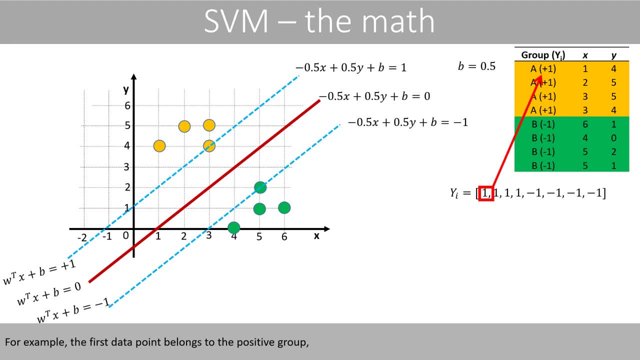 For example, the first data point belongs to the positive group, whereas data point number 5 belongs to the negative group. This is just another way to tell if the data point in our training data belongs to group A or B. The classification in support vector machines is usually defined like this: 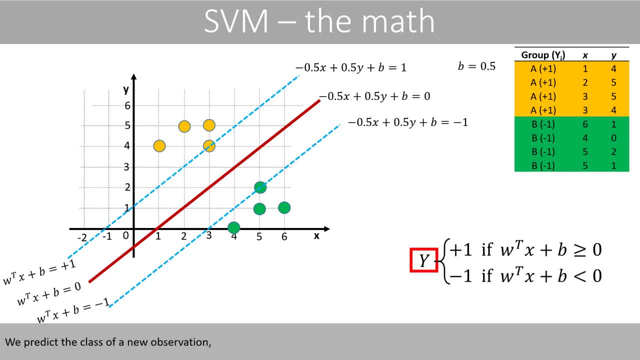 We predict the class of a new observation to belong to the positive group. If it is a positive group, if it is above or on the hyperplane. in our example, if the data point is below the hyperplane, we predict that the new observation belongs to the negative group. 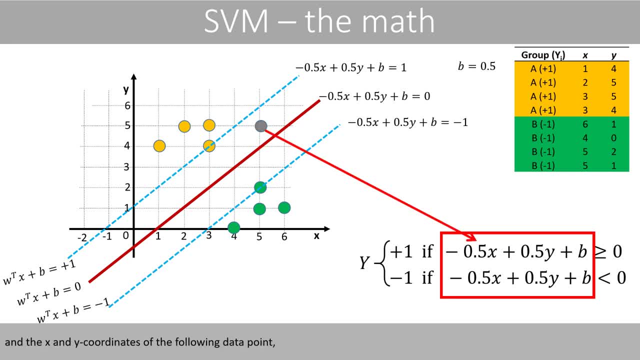 If we plug in the equation of our hyperplane and the x and y coordinates of the following data point, we would see that the calculation would result in a value larger than 0, which means that we will predict that the data point belongs to the positive group. 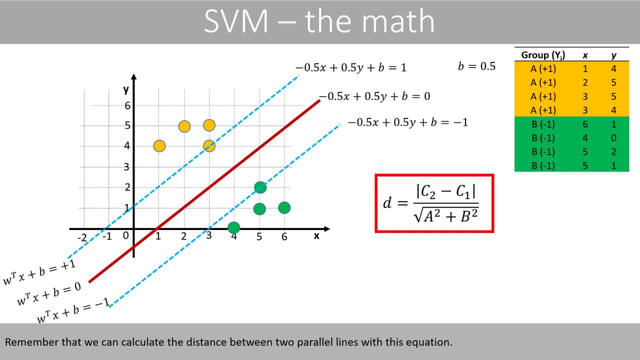 Remember that we can calculate the distance between two parallel lines with this equation and in a special case where we have normalized equations like this, We can simplify the equation to this, because the absolute difference between the constant terms is always 2.. Remember that w is a vector of a and b in our example. 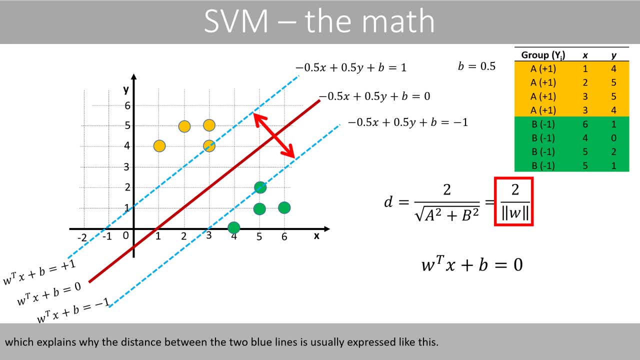 which explains why the distance between the two blue lines is usually expressed like this: If there is a line that can separate the two groups completely, a support vector machine tries to find the optimal values of a and b so that the distance between the two blue lines is maximized. 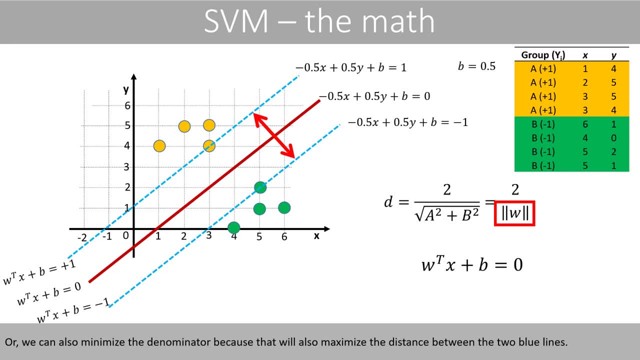 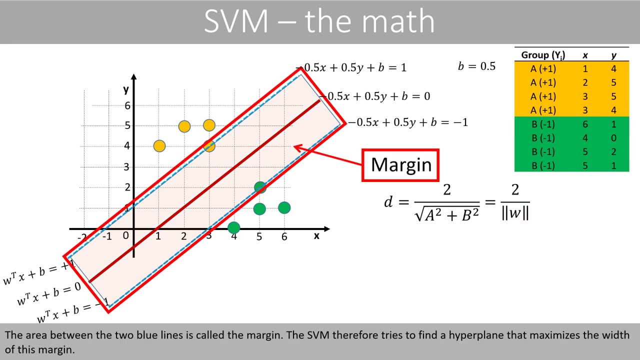 Or we can also minimize the denominator, because that will also maximize the distance between the two blue lines. The area between the two blue lines is called the margin. The support vector machine therefore tries to find a hyperplane that maximizes the width of this margin. 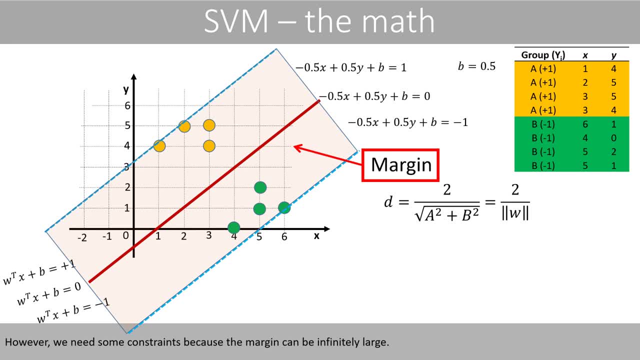 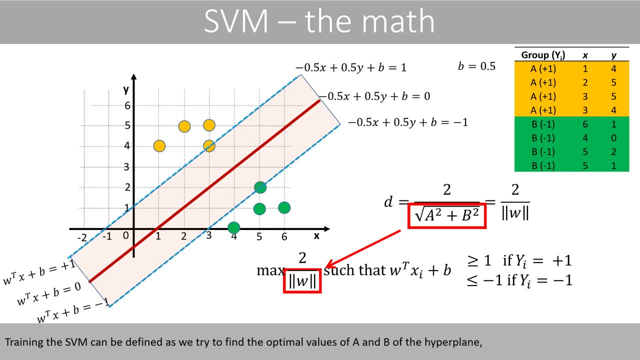 However, we need some constraints because the margin can be infinitely large. Training the support vector machine can be defined as we try to find the optimal values of a and b of the hyperplane so that we maximize the margin, So that our data points that belong to the positive group. 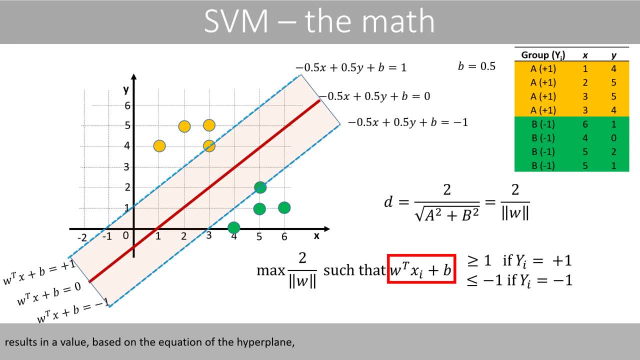 results in a value based on the equation of the hyperplane that is equal to or greater than 1, and that the data points that belong to the negative group results in a value that is equal to or less than negative 1.. This means that the margin should not span beyond the data points closest to the hyperplane. 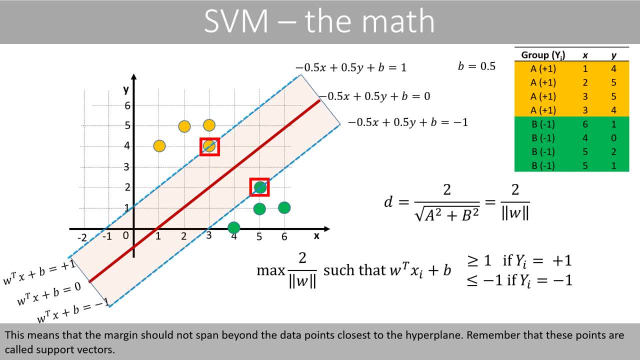 Remember that these points are called support vectors. Let's see what value we get if we plug in the x and y coordinates of this data point in the equation of our hyperplane, Since this data point represents the support vector that is on the blue line below the hyperplane. 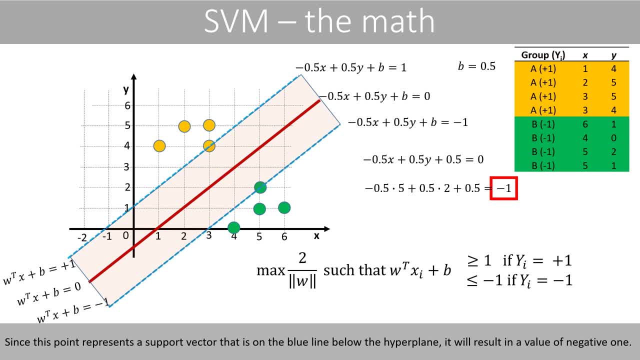 it will result in a value of negative 1.. The width of the margin is therefore constrained so that it cannot span beyond the support vector. If the hyperplane can separate the two groups completely, Similarly, the line that defines the boundary above our hyperplane cannot be further away. 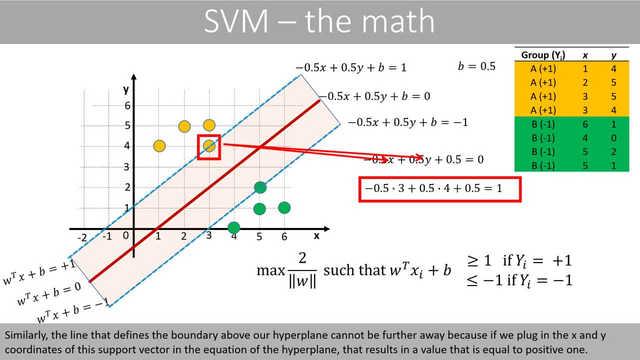 because if we plug in the x and y coordinates of this support vector in the equation of the hyperplane, that results in a value that is equal to positive 1.. A data point that is further away will result in a value that is larger than positive 1,. 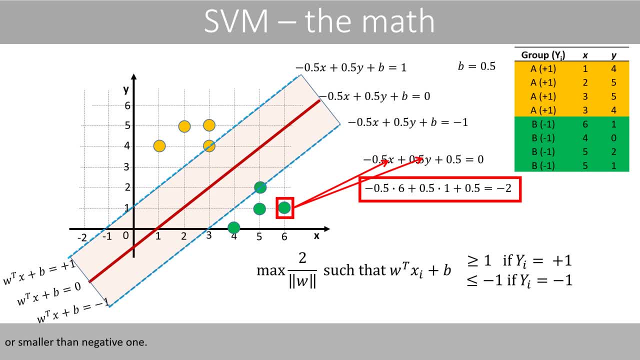 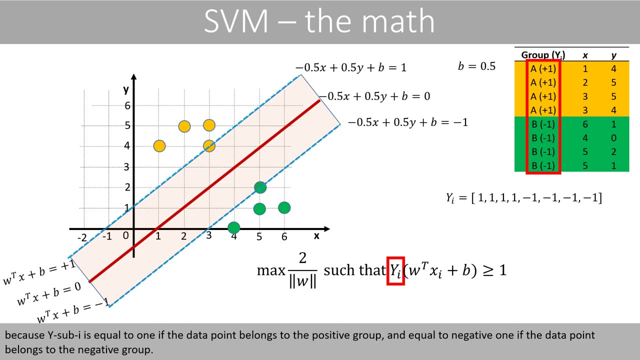 or smaller than negative 1.. We can simplify this equation a bit if we multiply the equation by y sub i, because y sub i is equal to 1 if the data point belongs to the positive group and equal to negative 1 if the data point belongs to the negative group. 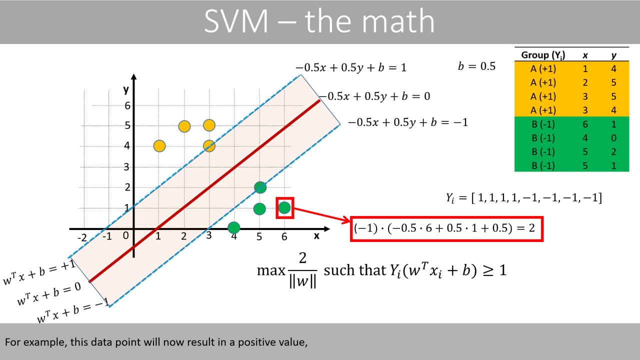 For example, this data point will now result in a positive value because we now multiply by negative 1, since this data point belongs to the negative group. Note that this type of problem is applicable only when the data can be fully separated by the hyperplane. 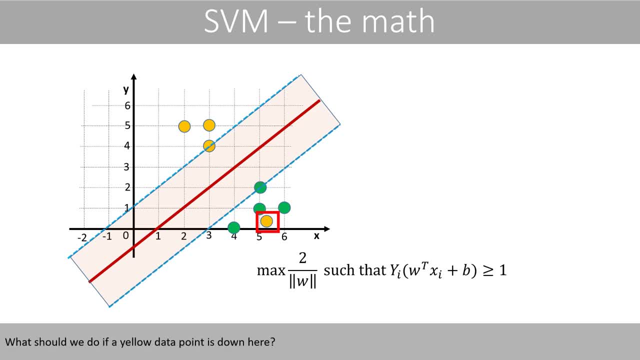 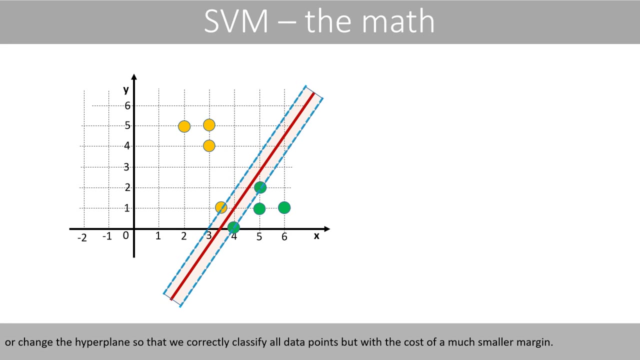 So what should we do? if a yellow data point is down here Or here, We can either accept that the data point will be incorrectly classified or change the hyperplane so that we correctly classify all data points, but with the cost of a much smaller margin. 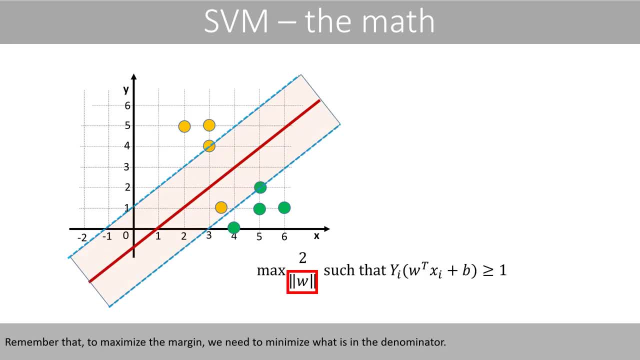 Remember that to maximize the margin, we need to minimize what's in the denominator. We can see this as we minimize only the denominator. For computational reasons, we usually express the term like this And to allow for misclassifications, we can add this term: 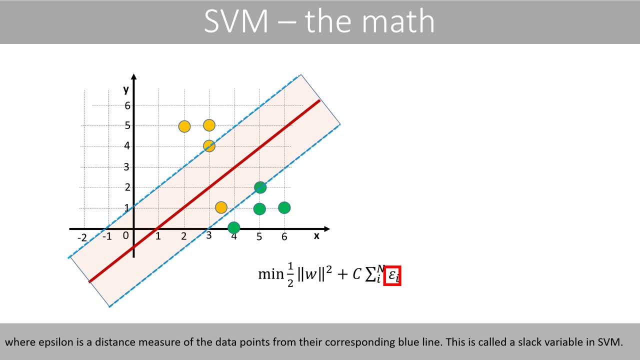 Where epsilon is the distance measure of the data points from their corresponding blue line. This is called a slack variable in support vector machines. In this example, there is only one data point that is incorrectly classified because it is on the wrong side of the hyperplane. 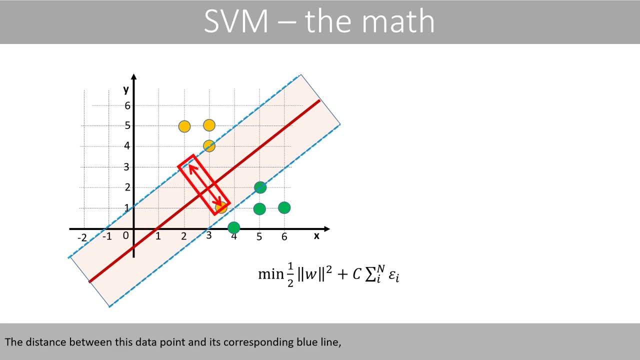 The distance between this data point and its corresponding blue line can be described by the following equation. Remember that the width of the margin can be calculated by the following formula: Whereas half the width of the margin, which is the distance between one of the blue lines and the hyperplane. 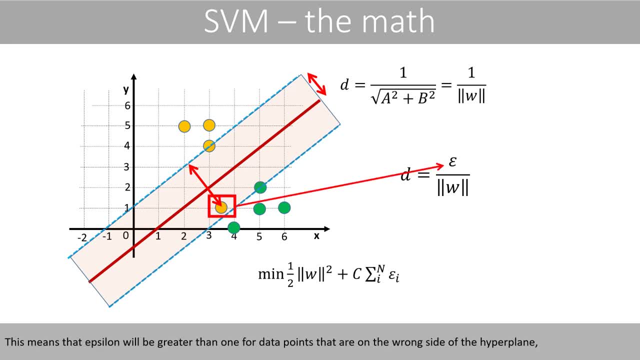 is calculated like this. This means that epsilon will be greater than 1 for data points that are on the wrong side of the hyperplane, Whereas a data point within the margin, but on the correct side of the hyperplane, will have an epsilon value that is between 0 and 1.. 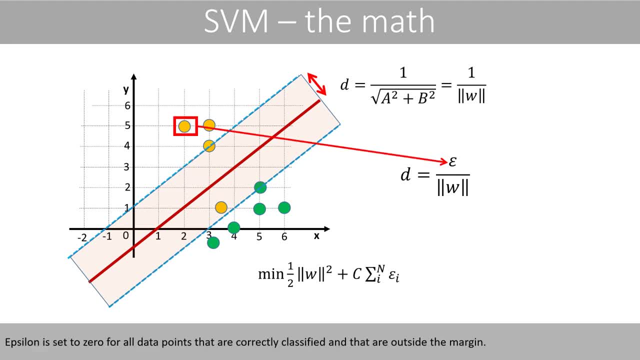 Epsilon is set to 0 for all data points that are correctly classified and that are outside the margin. Note that this point is now also considered as a support vector, because it will influence the orientation of the hyperplane like this for a certain value of c. 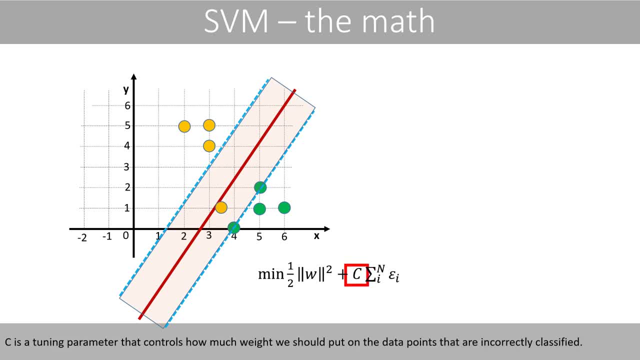 c is a tuning parameter that controls how much weight we should put on the data points that are on the margin. If c is small, we will get a large margin where we put little weight on data points that are misclassified. This will result in a so-called soft margin support vector machine. 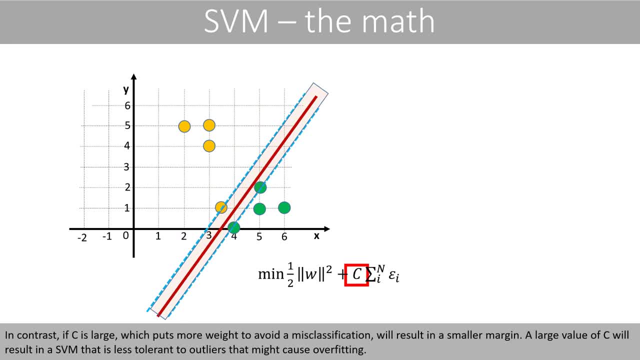 In contrast, if c is large, which puts more weight to avoid misclassification, will result in a smaller margin. A large value of c will result in a support vector machine that is less tolerant to outliers that might cause overfitting. A value of c can be optimized by using, for example, cross-validation. 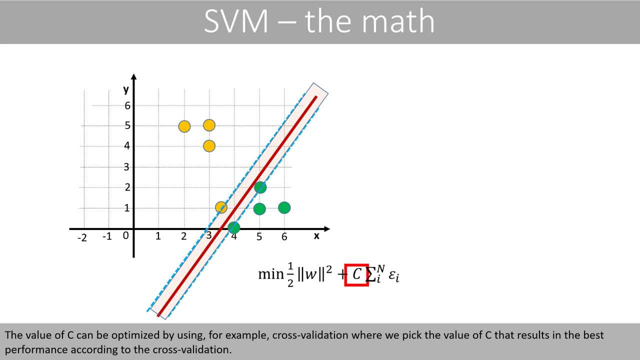 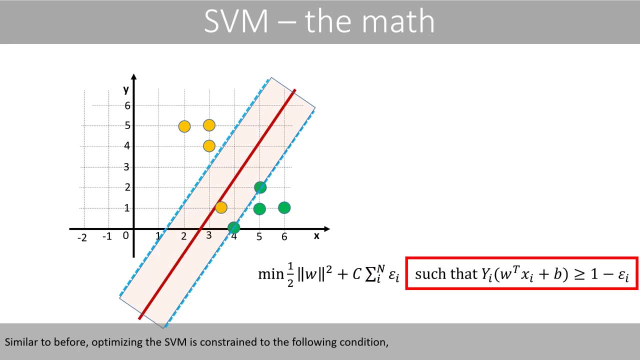 where we pick the value of c that results in the best performance according to the cross-validation. Similar as before, optimizing the support vector machine is constrained by the following condition: Where all correctly classified data points outside the margin should result in a value equal to or greater than 1,. 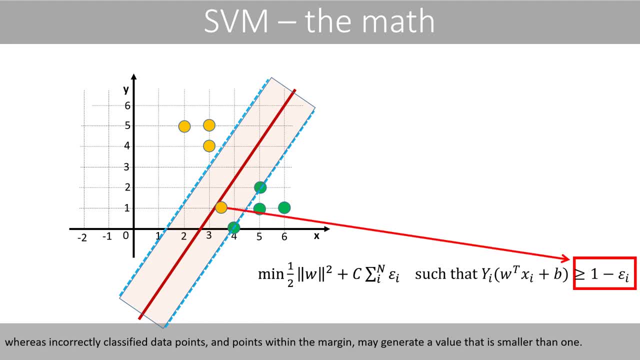 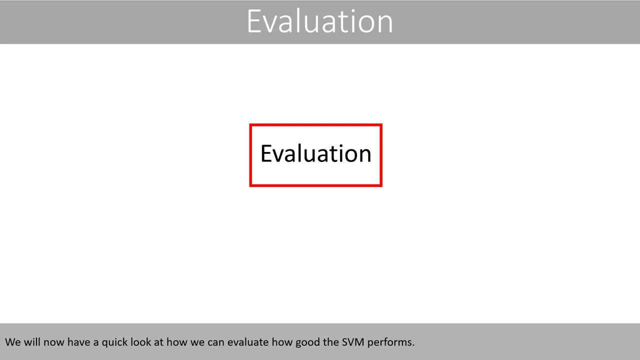 according to the hyperplane, Whereas incorrectly classified data points and points within the margin may generate a value that is smaller than 1.. We'll now have a quick look at how we can evaluate how good the support vector machine performs. Suppose that we have trained our support vector machine. 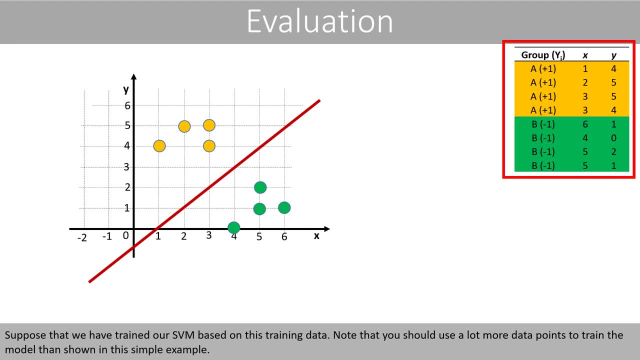 based on this training data. Note that you should use a lot more data points to train them all than shown in this simple example. Let's say that the support vector machine has optimized the coefficients to these values of our hyperplane according to the function we saw earlier. 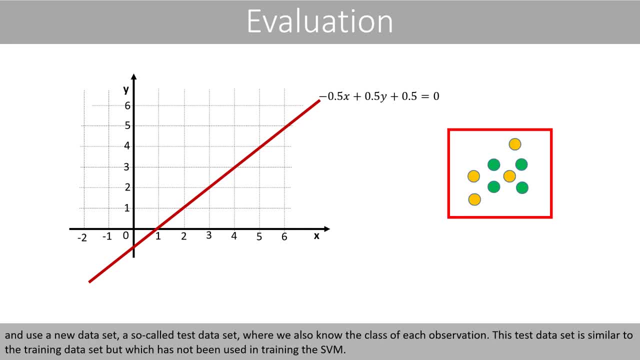 We now remove the training data and use a new dataset, a so-called test dataset, where we also know the class of each observation. This test dataset is similar to the training data, but which has not been used in training the support vector machine. We then place the test dataset in the plot. 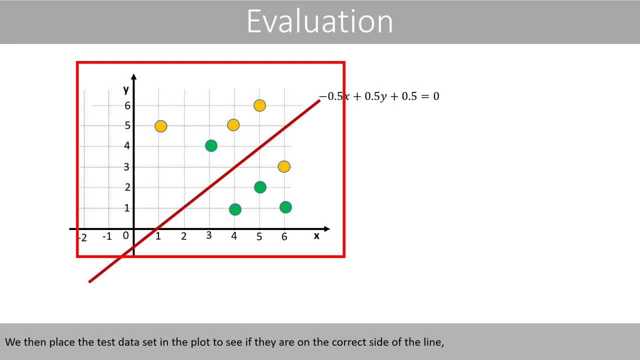 to see if they are on the correct side of the line. We'll simply plug in their coordinates in the equation of the hyperplane to see if they result in positive or negative values. We see that we make two incorrect predictions because these two data points 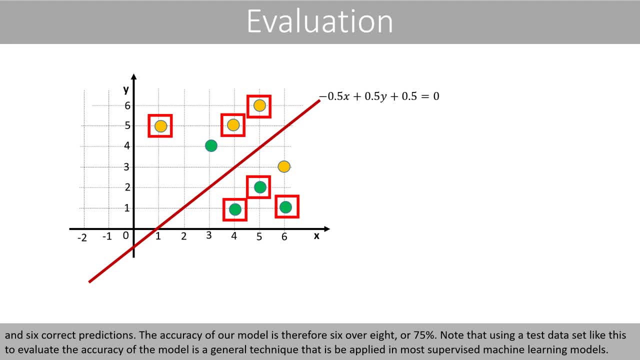 are on the wrong side of the hyperplane And six correct predictions. The accuracy of our model is therefore 6 over 8, or 75%. Note that using a test dataset like this to evaluate the accuracy of the model is a general technique that is applied. 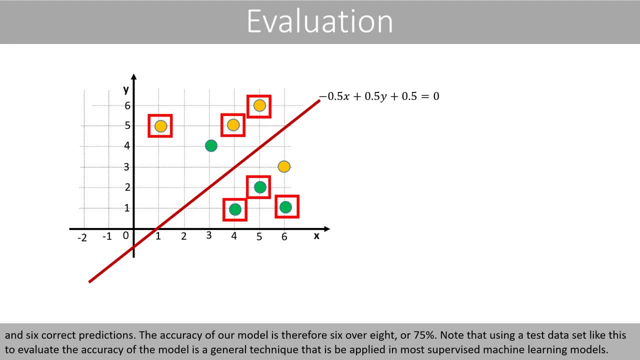 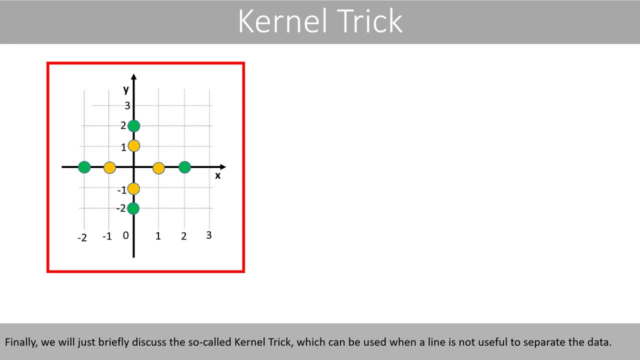 in most supervised machine learning methods. Finally, we'll just briefly discuss the so-called Kerner trick, which can be used when the straight line is not useful to separate the data. For this type of data, a straight line does not make a good job. 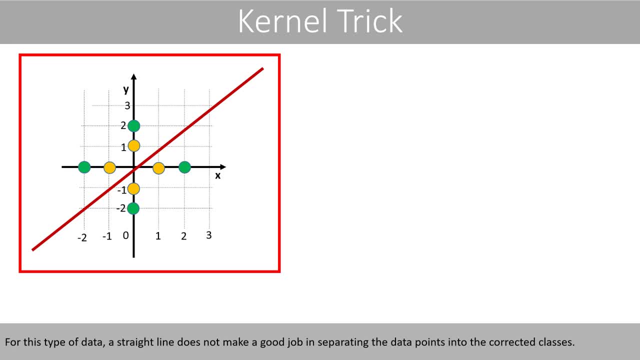 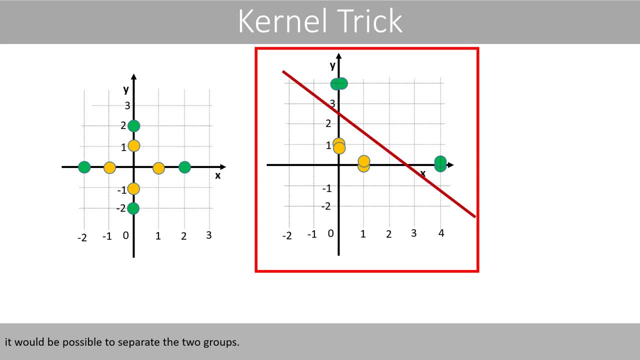 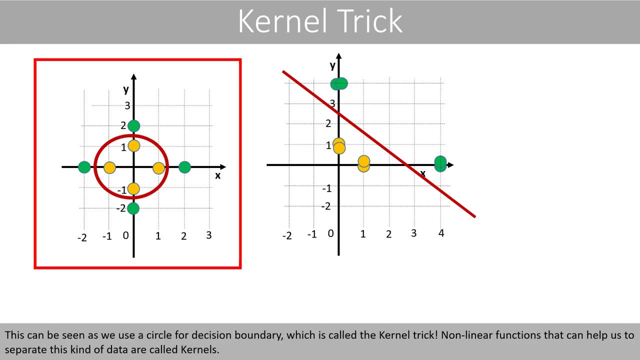 in separating the data points into the correct classes. If we would, for example, square the coordinates of the data points, it would be possible to separate the two groups. This can be seen as we use a circle for decision boundary, which is called the Kerner trick. 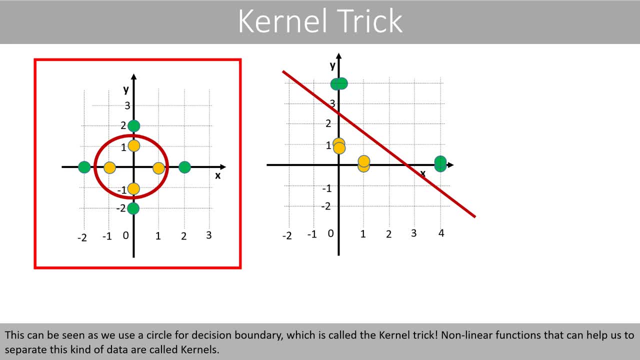 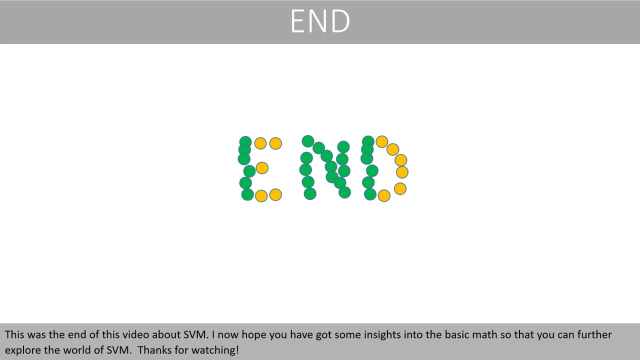 Some linear functions that can help us to separate this kind of data are called kernels. This was the end of this video about support vector machines. I now hope that you have got some insights into the basic math so that you can further explore the world of support vector machines. Thanks for watching. 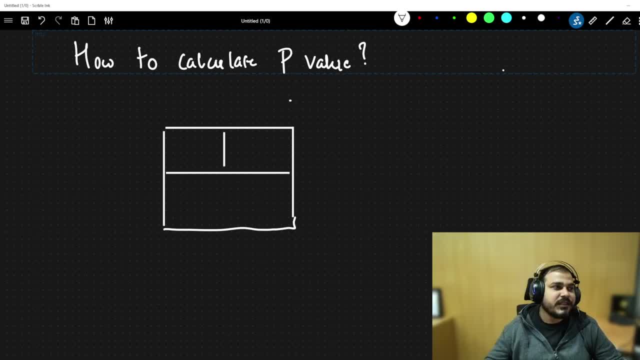 Hello all my name is Krishnayak and welcome to my YouTube channel. So, guys, today, in this particular video, we are going to see about how to calculate p-value. Now, many people have a lot of confusion with respect to p-value- significance value- and this is specifically related to. 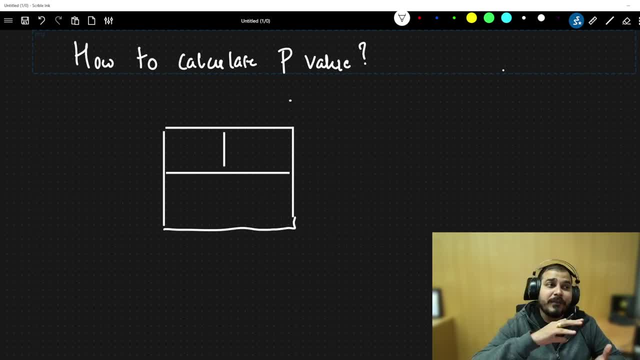 hypothesis testing, and sometimes I also feel a lot of confused when I'm again revisiting the concept or when I'm teaching somewhere. you know at the same point that same thing will not strike and probably I have to revise again and again. So in this particular video I will try to solve. 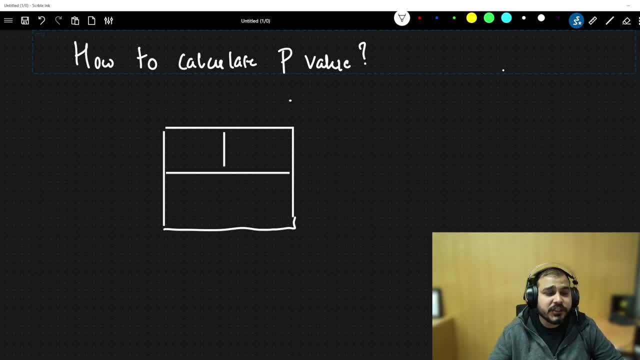 a problem and also try to show you, with Python programming language, how to calculate p-value and what is the importance of p-value and what is the difference between p-value and significance value. So first of all, let's go ahead and let's try to see this particular concept of p-value.